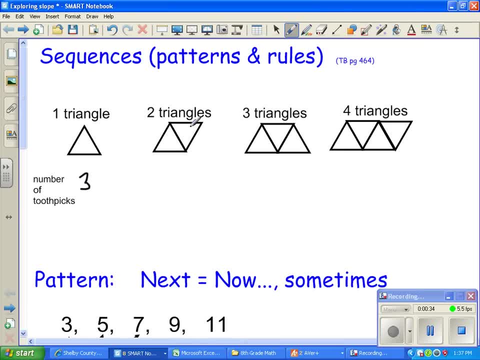 Okay, and the second one. I have two triangles, but how many toothpicks did it take to make that? It took five. In your book they count the illustrations a little better For three triangles. how many toothpicks did it take? 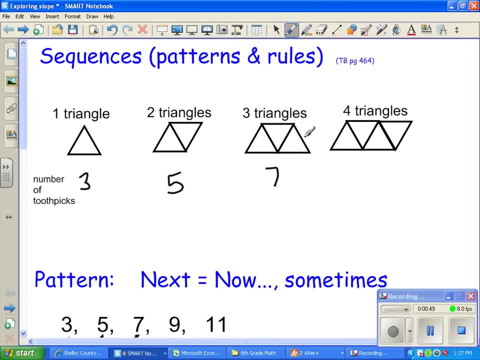 Somebody said seven, We count one, two, three, four, five, six, seven, And for four triangles we get nine. Now we could continue this pattern. If we were out for five triangles, what would it be For six, for seven, for eight? 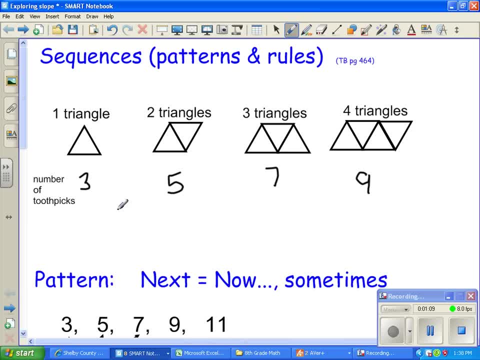 In doing so, we're trying to find the pattern. Is there a pattern that occurs? What do you notice? It looks like I'm adding two each time. Okay, So we can say: if you remember from last year, we're adding two. 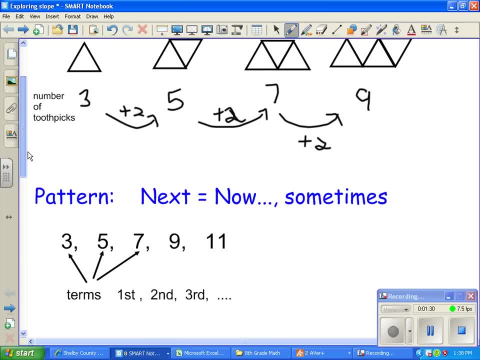 So we can say: if you remember from last year, we're adding two. So we can say, if you remember from last year, we're adding two. So we should have made sure that we had said it as a next equals now. 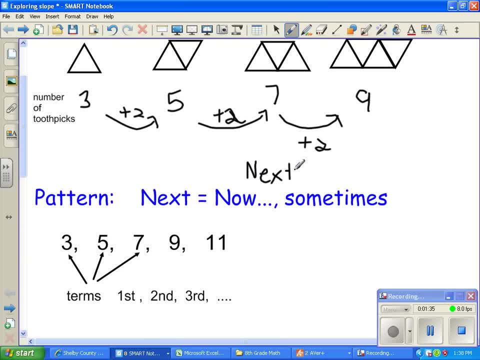 So this one would be next equals now. and what Plus two? Okay, and that's stating the pattern. Now, not all patterns have a next equals now. There may be a pattern where it goes one, then it goes two, then you add three, then you add four. 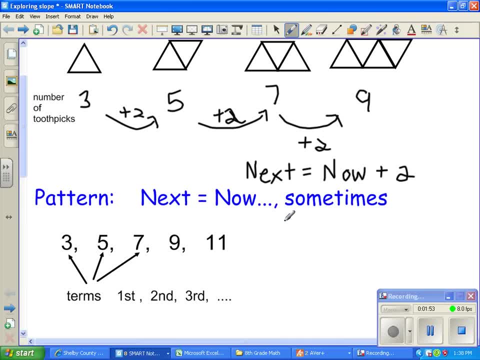 Okay, but what we're looking at now is we're looking at a special pattern in which you either add or subtract the same number each time, and that can be stated as a next equation now. now, when you're given a pattern like this, I'm going to make a suggestion. 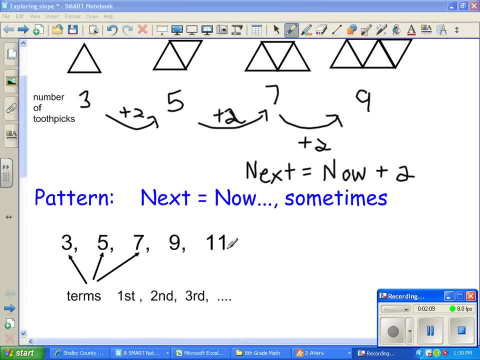 that's really, really huge. if you do this, it'll make your life so much easier when you're trying to find not just the pattern, but the rule. I have a sequence of numbers three, five, seven, nine, eleven- same sequence or pattern that we had up here. instead of writing going across horizontally, let's make them into a 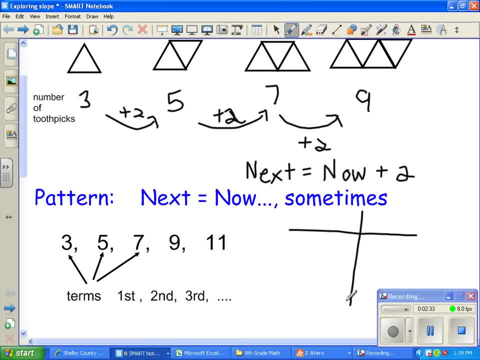 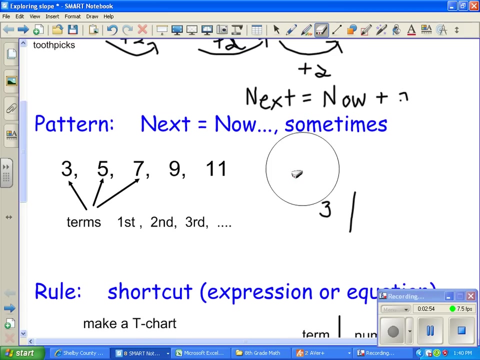 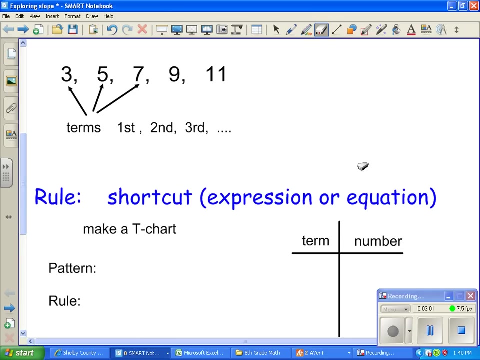 t-chart, okay, with the end representing the term number: first, second, third and so forth. okay, I think I have this down later on, so let's write. let me go down to that one. each term has a place. three is in the. it's the first term, so you can kind of call it the first place. second term, third term. 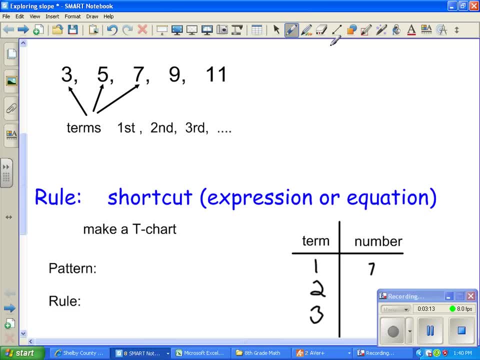 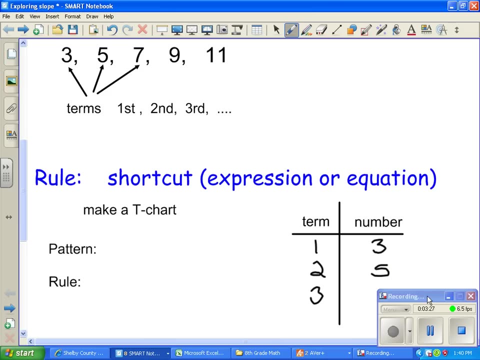 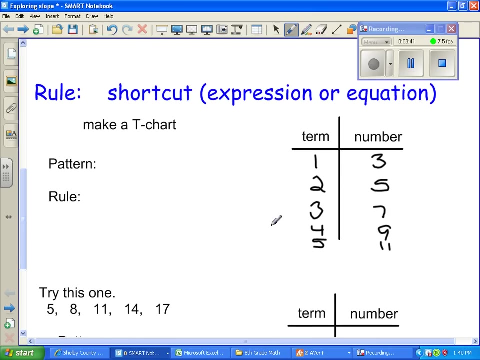 and so forth, a term, or you can call it in: okay, what's the second term? five. what's the third term? fourth, nine and the fifth is 11. okay, now we have already found the pattern correct. that's going this direction. how does each change each time? that's the pattern and you notice we add to each time the. 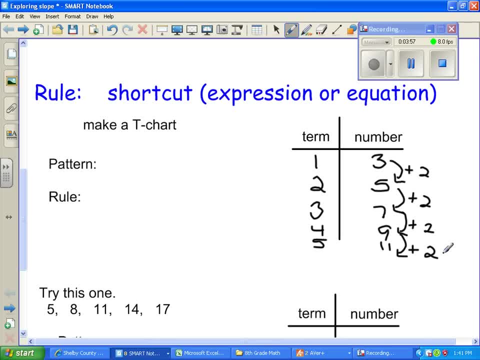 change each time. that's the pattern and you notice we add to each time the change each time. that's the pattern and you notice we add to each time the. you know, I kind of like shortcuts. I can't like to see if I could find a shortcut, so if I want to know what the 20th term was, in other words, if I have. 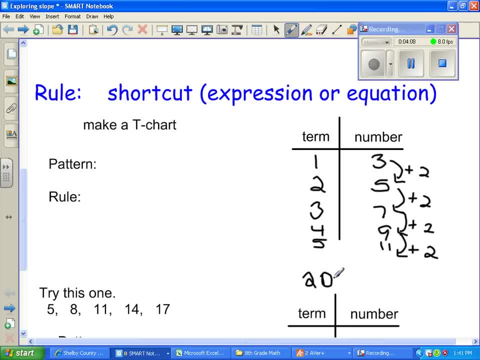 20 triangles. how many tooth picks am I going to need? and I sure would like to do it some way other than counting down six, seven, eight, nine, ten, all the way down. so what is it that we're going to find in order to get that shortcut know? 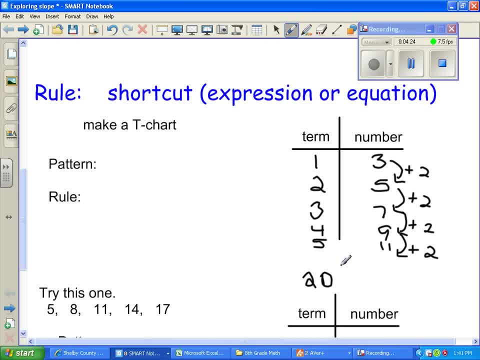 what that's called, Mary. you could find that in. it's called a second layer pattern. I'm going to find the rule Now. the rule goes from term number to your number. Okay, in other words, if I go to the second, what do I do to this 2 to get a 5?? 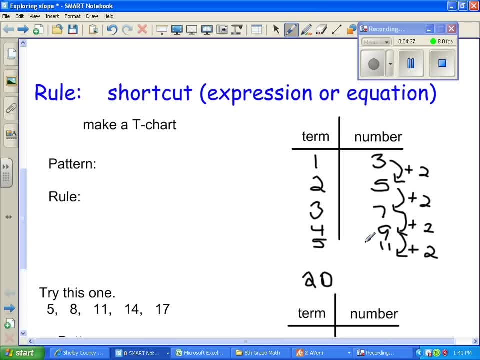 What do I do to 3 to get a 7?? What do I do to 4 to get a 9, and so forth? I want you to think about that just for a minute, If you think you've come up with a rule that would apply. 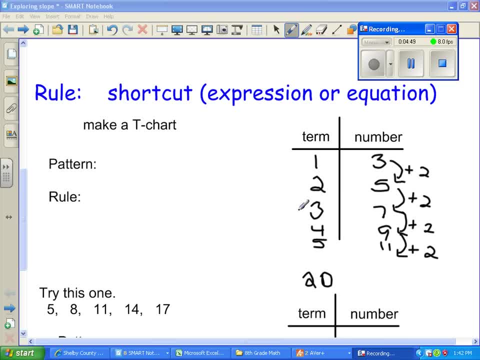 why don't you share it with your partner and see if they agree? Okay, what are you noticing, Crystal? She says: I'm taking my term number times 2 and then adding 1.. Let's try it: 1 times 2 is. 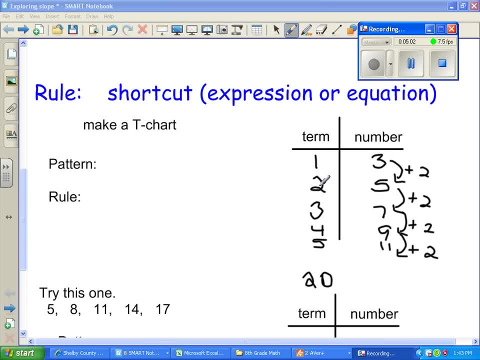 Plus 1 is 2 times 2 is Plus 1 is 3 times 2 is Plus 1 is Wow, it must be working. So 20 times 2 is Plus 1 would be 41.. 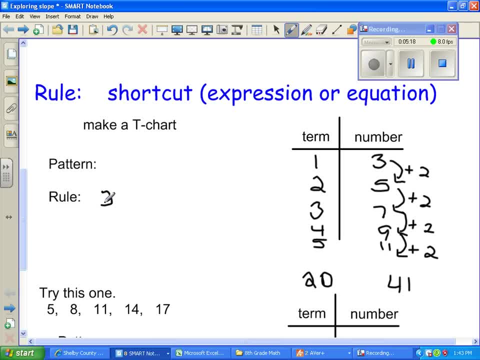 So my rule that I'm going to refer to is: 2 times 2 is N plus 1.. Where N is my term number. The pattern was: your next equals now statement. Now, it doesn't always have to be a next equals now statement. 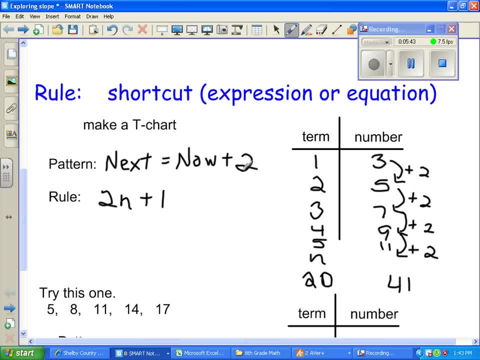 And the pattern could have been a plus 1,, plus 2,, plus 3, and then you put dot dot dots saying that that pattern continues, And then we find the rule. Now, do you notice anything about that rule? 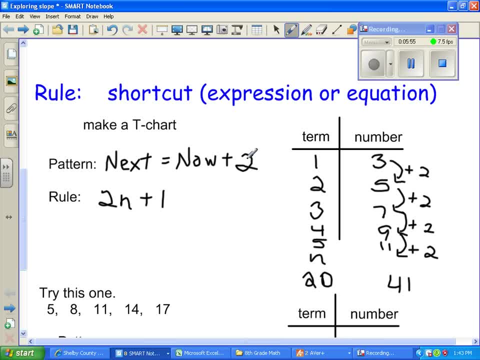 and the pattern that have something in common, Or maybe something you might have a clue about. What did you notice, Taylor? Okay, the pattern was a 2.. So do you think that always your rule might involve a 2?? Well, if it's not. 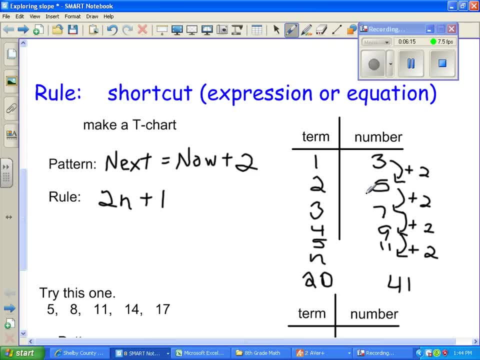 there's not a direct connection, that's a place to start. Okay, I'm not going to say it always works, but it's always a good place to start. In other words, if I can say to myself: okay, 1 plus 2 is 3,. 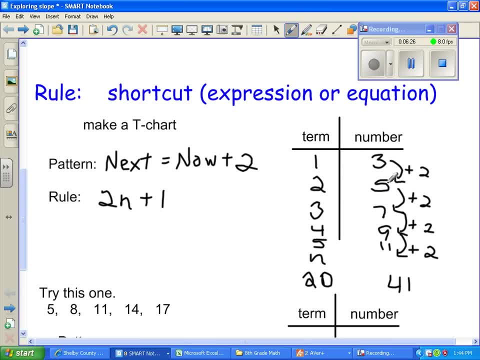 but not. 2 plus 2 doesn't give me 5.. Okay, that's not going to work. So let me try multiplying: 1 times 3 is 3, but 2 times 3 isn't 5.. Okay, that's not working. 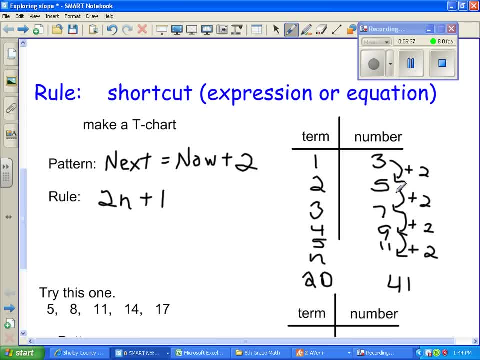 So that tells me that's probably a 2-step rule. It's going to have 2 steps that take place, And we found out that it did. So try using the 2 or taking 2 times your number and then see how far off you are. 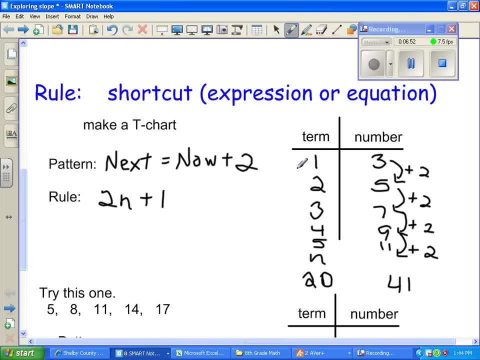 Okay, So I tried 2 times 1, and I got 2,, but I'm still how many away from 1 away? 2 times 2 is 4, but I'm still 1 away. 3 times 2, 6,, but I'm still 1 away. 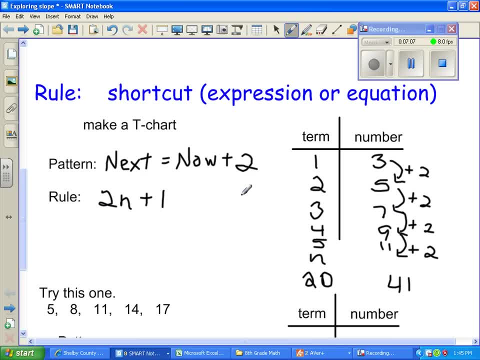 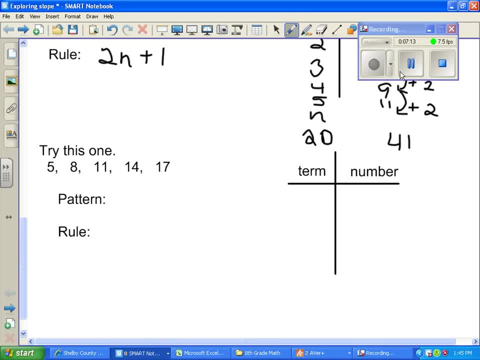 So then that tells me that I'm going to take 2 times n plus 1.. Now, do you think that always works? Now, let's try it. Write this one down in your handy dandy and try it. See if you can come up with a pattern and the rule. 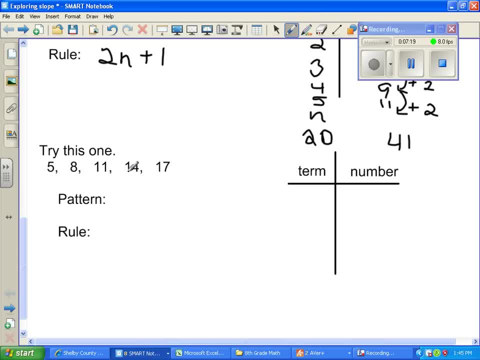 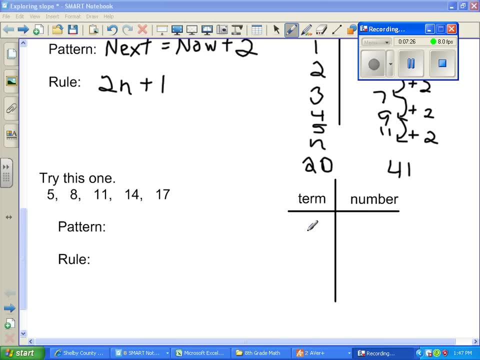 5,, 8,, 11,, 14, and 17.. First, okay, Okay, your first step is: I'm going to transfer it into a T-chart. My first term was 5.. My second term was 8.. 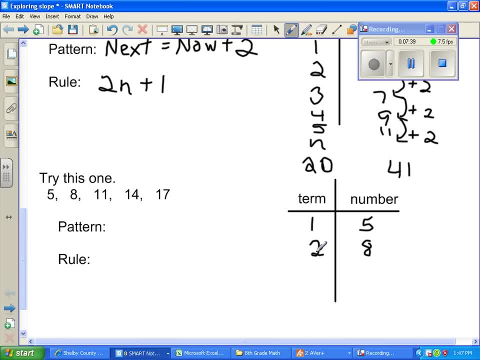 And oftentimes they'll be just listed as numbers, so you have to translate that into which term. The third term is 11.. The fourth term is 14. And the fifth term is what? 17.. Okay, the first thing is: let's look for a pattern. 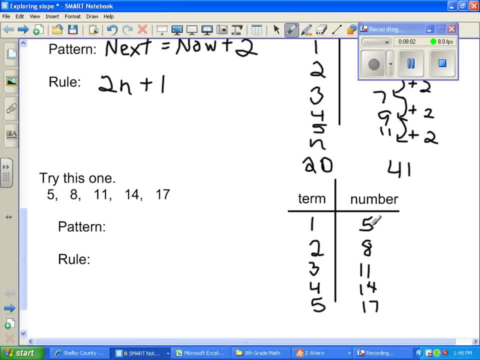 Mary, what did you do to find the pattern? Okay, I'm looking at your numbers and just seeing what are they doing. In other words, from here, what am I? where am I going? each time I am adding 3.. 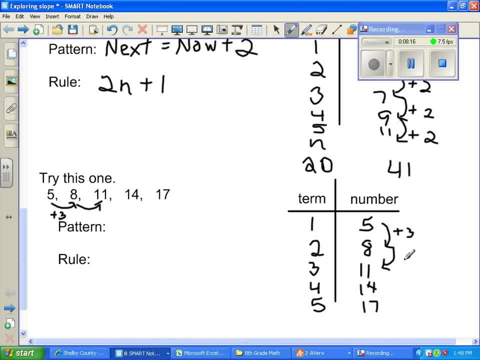 Okay, so I can say that that's my pattern. Okay, To add 3.. To add 3.. Can I state that in a next equals now, Yes, Next equals now plus 3.. If you couldn't put it in a next equals now, like, let's say, it went up 1 and then it went. 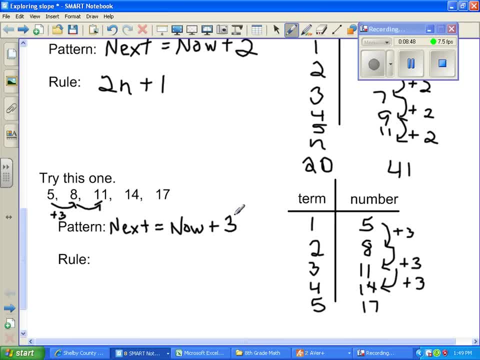 up 2, then 3.. You would put a plus 1, comma plus 2, comma plus 3, comma. dot dot dot, Because you've given enough to show us what the pattern is. Okay, but this clearly is a plus 3 every time. 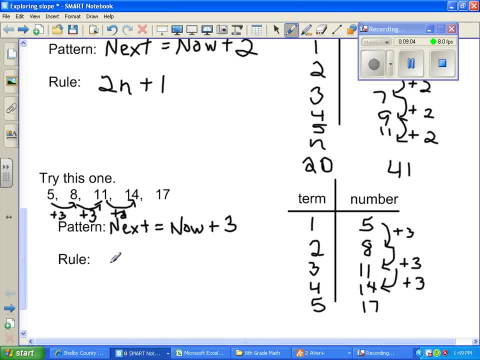 Okay, now let's take a look at your rule Because, remember, if we find that this happens sometimes, that helps us with our rule. Let's see is there anything I could do directly like 1 plus 4 gives you 5,. 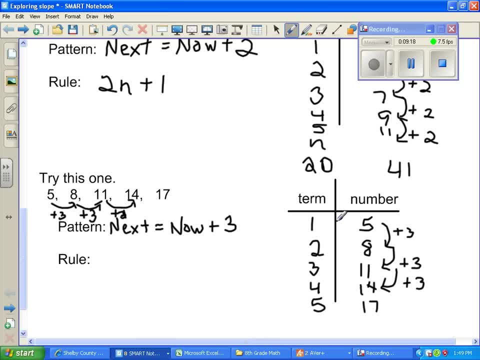 so it's 2 plus 4. 8, that's not working. is it Okay? 1 times 5, 5. Yes, but it's 2 times 5, 8.. Okay, that doesn't work. 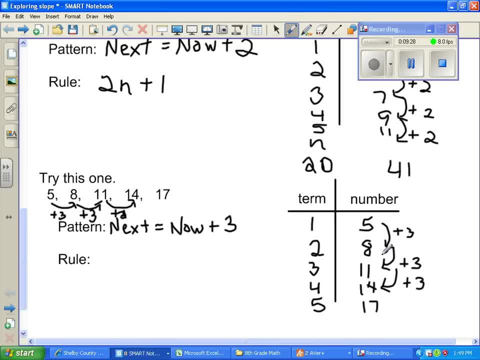 And that's where you need to start. You need to look to see: is there a direct relationship? There isn't. So what do you think, Jake? Okay, and what was your pattern 3.. So does it have anything to do with 3?? 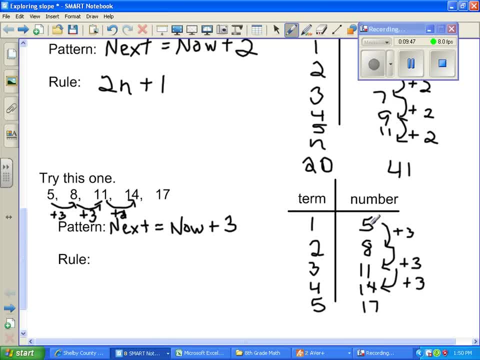 So try this: What's 1 times 3? And I'm 2 away from my goal? right? What's 2 times 3? And I'm 2 away from my goal? Hmm, what's 3 times 3?? 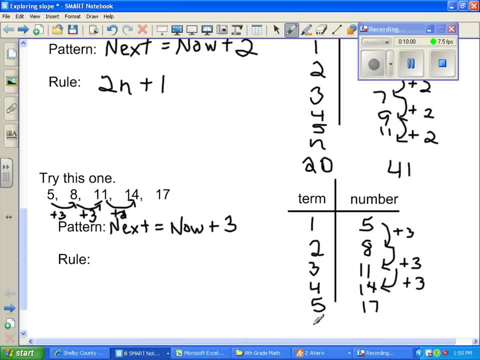 And I'm 2 away from my goal. So we can say that the rule: if I put an N here I'm going to have to take 3 times N and then do what to it Plus 2.. How many had that? 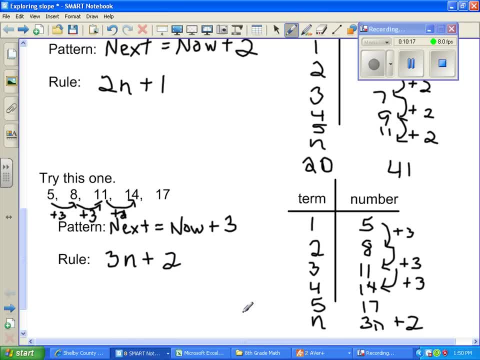 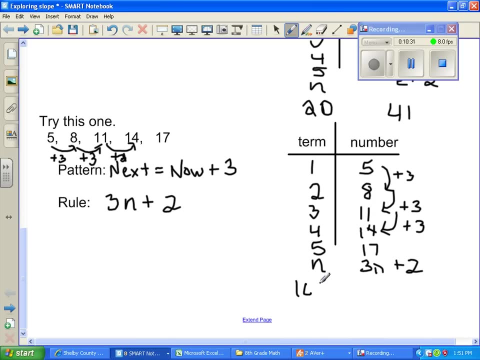 Good. So this helps us. if I want to ask: okay, if I have 100 terms, what would be the 100th term in this sequence? What would I do? Rochelle 3 times 100, which gives you 300, plus 2.. 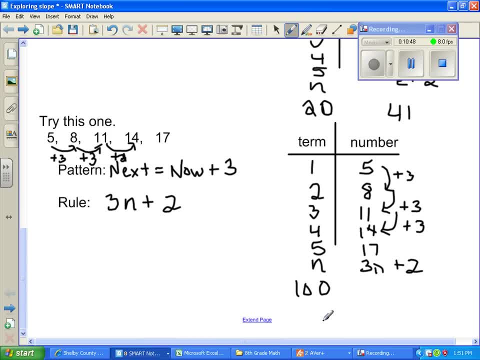 That's right, You get 302.. So that saves me from having to make that whole long, boring list. is if I can arrange it and find a rule. Yes, Shawn, Do you always use this? I'm saying a lot of times it could be a key. 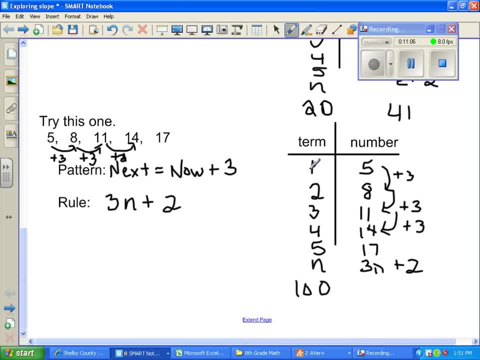 There are some times that, no, that doesn't help you. One clue is, Shawn: if you're going to have term 1,, 2,, 3,, 4, 5, it works. Sometimes they have other numbers than 1,, 2,, 3,, 4, 5.. 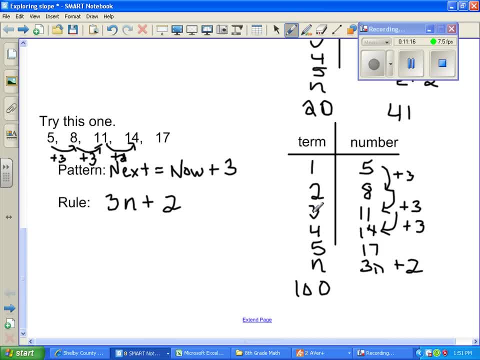 That's right. So then it doesn't always work. They give them to you, okay. When we get to plotting ordered pairs, it oftentimes does not work. Shawn, Okay, if they're just giving you a set of numbers, then you can use the first second. 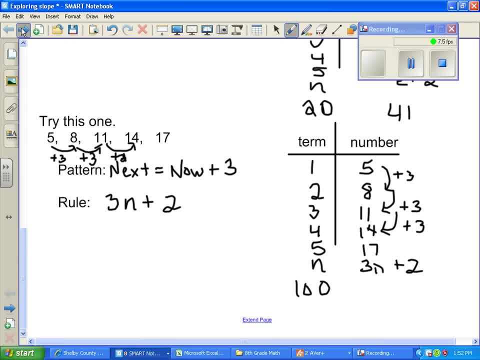 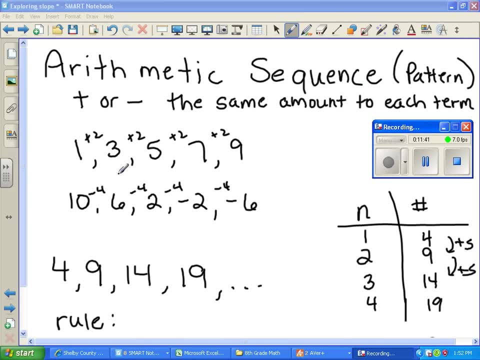 third, fourth, fifth, and you put them in that order. What's this kind of pattern called? This kind of pattern is called an arithmetic sequence, The one that we just looked at. It's called an arithmetic sequence. Arithmetic sequence or pattern. 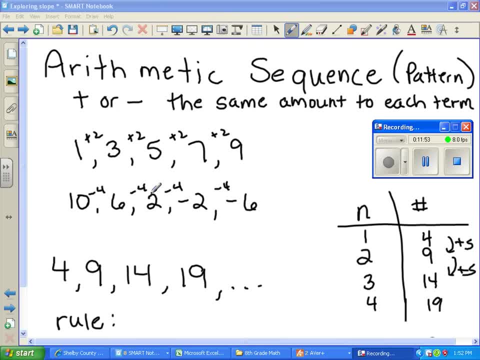 An arithmetic sequence is when you add or subtract the same amount to each term. It's a special pattern or sequence once you add or subtract the same amount to each term. For instance, if I have the pattern 1,, 3,, 5,, 7,, 9,, I would be adding 2 each time. so 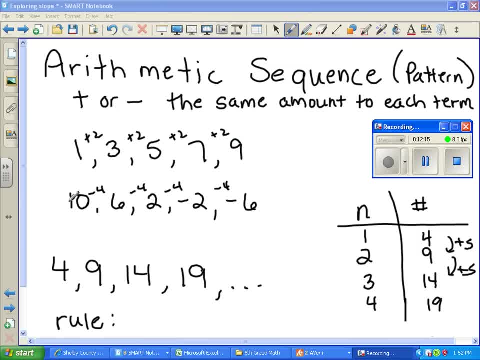 this one is an arithmetic sequence. If I had the example 10, 6, 2, negative 2, negative 6, I'm having to subtract 4 each time. Therefore, it too is also an arithmetic sequence. 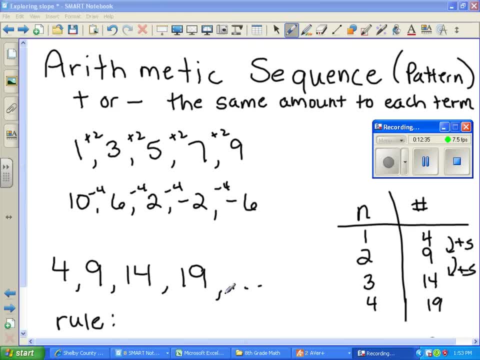 Now let's take a look at the pattern 4,, 9,, 14,, 19.. Let's see if there's a pattern and if there is a rule that we can apply. Remember the first one: It's a rule. The first thing, especially if you're looking for your rule, is to set it up using a T-chart. 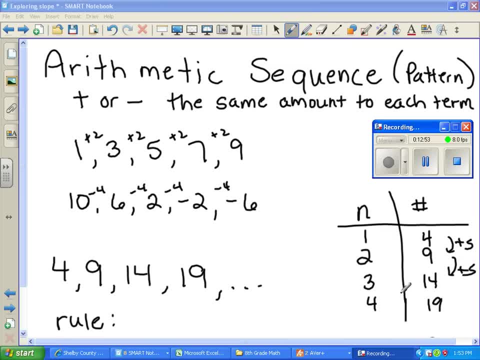 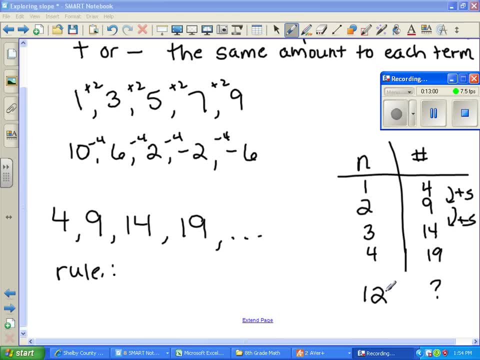 That's the key. If you want to try to find the rule, set it up in a T-chart. I'll give you a few minutes to work on that. I'm going to say I want you to try to find the pattern and then the rule in order to 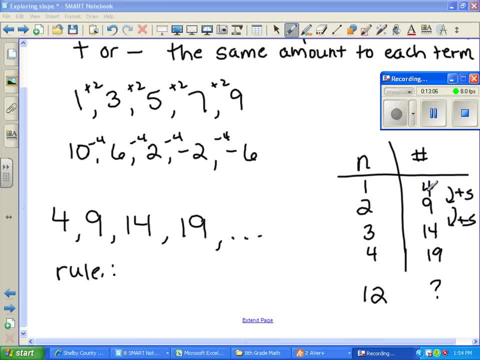 get us so that we know what the 12th term will. be All right, so I record: my first term was 4.. My second term is 9.. Third was 14. And fourth was 19.. Is there a rule to lift that up? 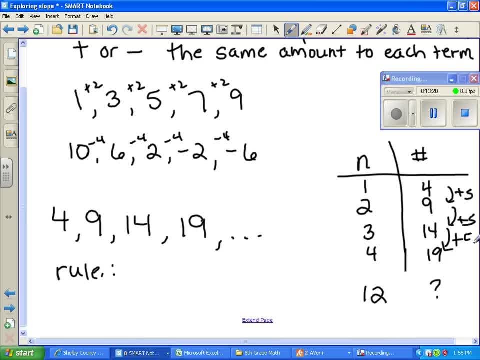 What pattern did you notice occurring? Shaun? Next equals. now, What are you doing each time? Just right here, How am I going from 4 to 9?? What am I doing? That's my pattern. I don't want the rule, quite yet. 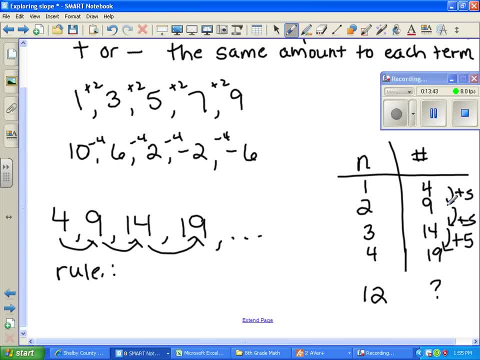 We're going to get to the rule 17. 16.. sorry, I can't add five. thank you, sorry. I was thinking this thing in my ear. it's even worse. my hearing aids don't work at near as well. okay, I need upgrade of.